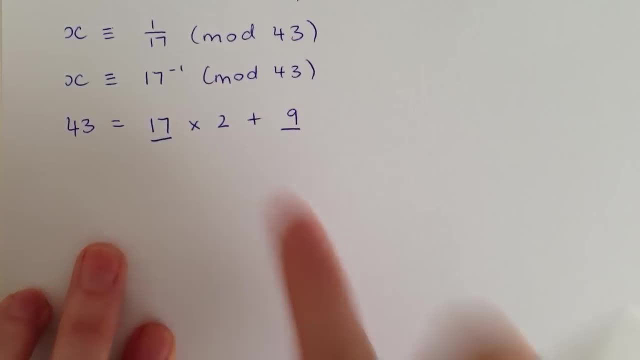 are the two that we want to bring down next time. So then we bring this 17 down, Bring the 9 down, And so that's times, what number? which is obviously 1, and then plus 8.. Underline them again, Okay, and then bring the 9 down, Bring the 8 down, And that's obviously. 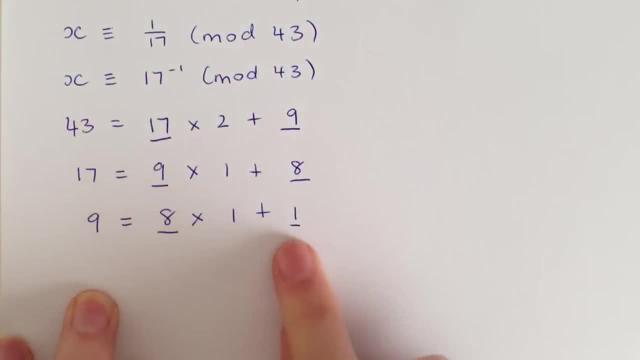 times 1 plus 1.. Now, when we get a 1 in this position, that means that the GCD of 43 and 17 is 1.. We can only ever find an inverse. We can only ever find an inverse number when this GCD is 1.. Otherwise, you can't do it. 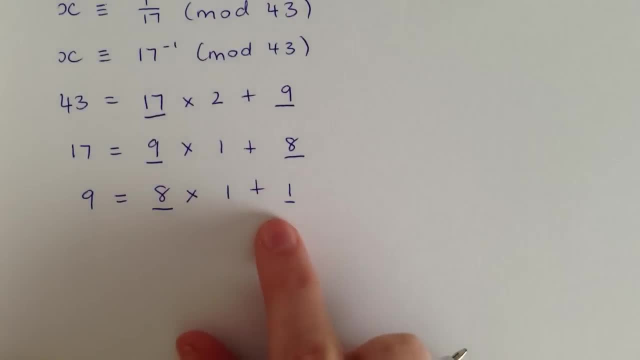 So in this case it is 1.. So we can continue. So now we want to move on to the extended Euclidean algorithm. So to do that, we want to write this term here in terms of sorry, this equation here in terms of 1.. So we want 1 equals now to get that on its own. we just 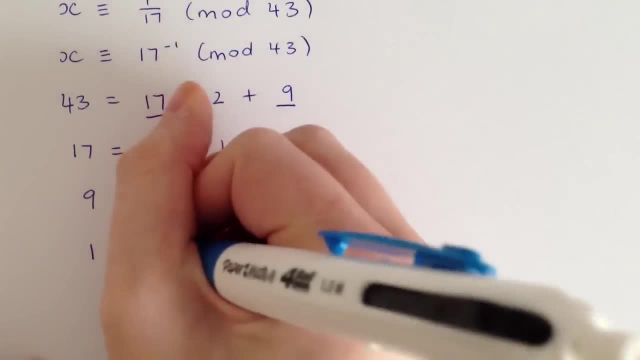 take this 8 times 1 over the other side, So we get 9 minus 8. And then it's times 1, but we can just leave it at that. And then we just take this 8 times 1 over the other side. So we get 9 minus 8.. And then it's times 1, but we can just leave it at that, And then we just take this 8 times 1 over the other side, So we get 9 minus 8.. And then we just 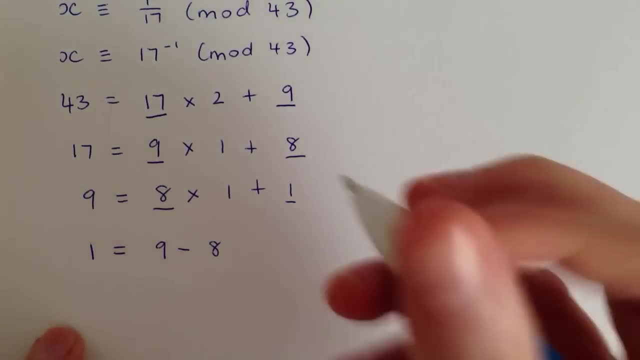 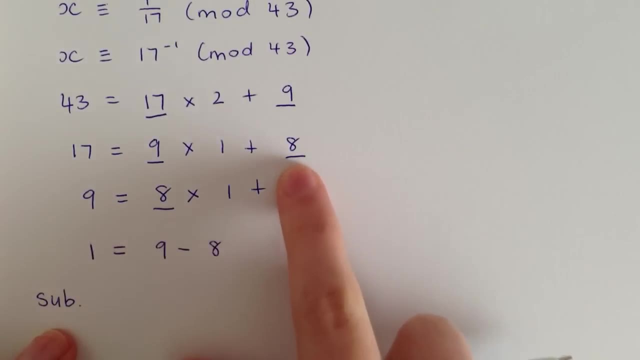 leave that off, because it's the same as saying 8.. Okay, so now we want to sub in. We've already worked with this equation, So we want to back up the Euclidean algorithm And we want to sub in this equation here. Now we want it. 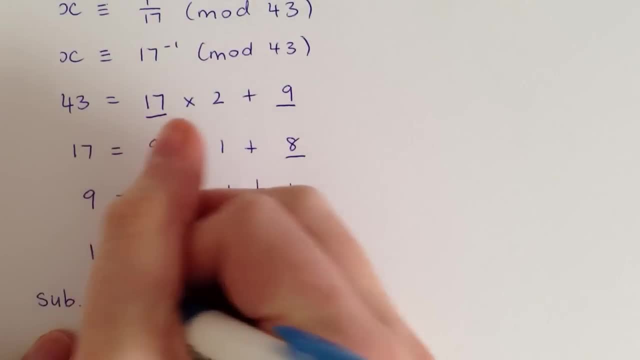 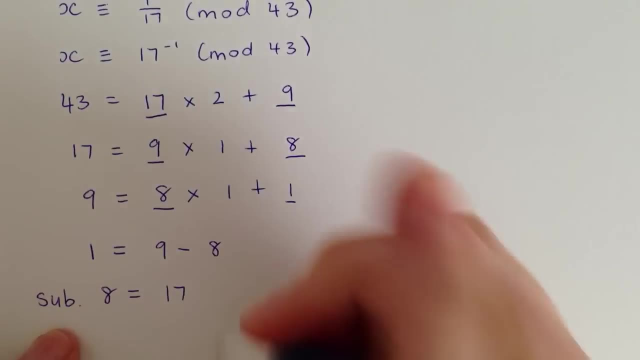 in terms of this number on the end, again So same as we did before. just take this 9 times 1 over the other side. So that gives us 17 minus 9 times 1 over the other side. So that gives us 17 minus 9, again times 1, but we can just leave it off because it's. 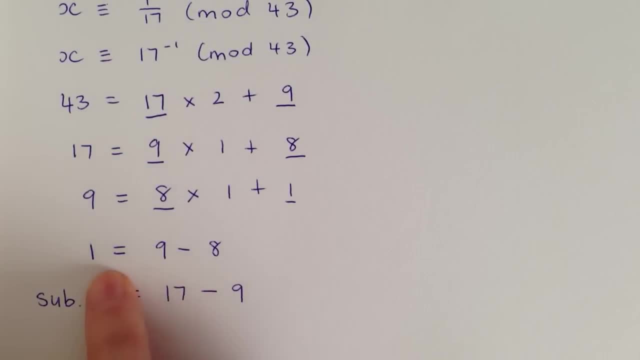 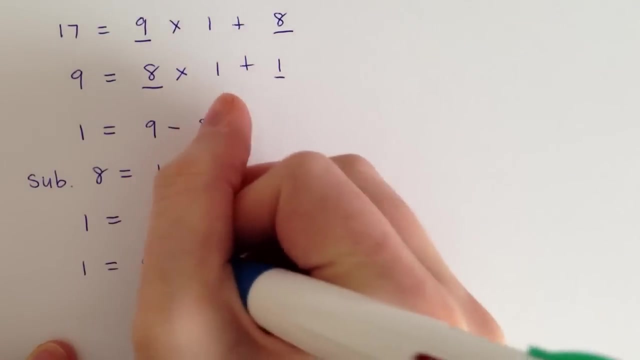 the same. So we want to sub this equation into this one just above it. So we'll get 1 equals 9 minus where there's an 8, you want to put this 17 minus 9.. And then we can just simplify that. A negative and a negative make a positive, And we can simplify that. 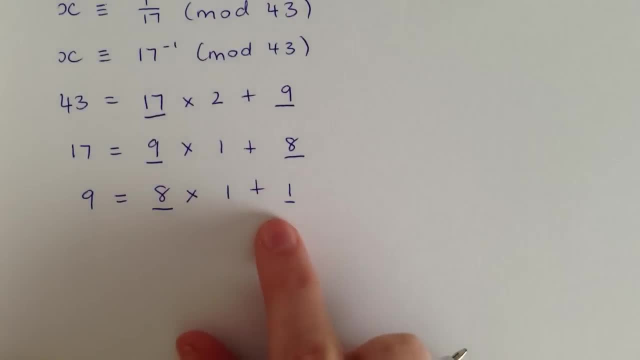 So in this case it is 1.. So we can continue. So now we want to move on to the extended Euclidean algorithm. So to do that, we want to write this term here in terms of sorry, this equation here in terms of 1.. So we want 1 equals now to get that on its own. we just 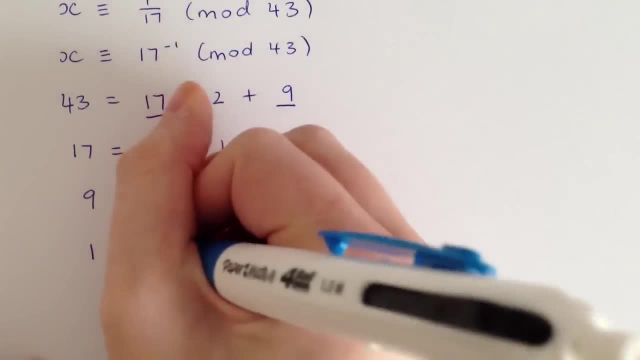 take this 8 times 1 over the other side, So we get 9 minus 8. And then it's times 1, but we can just leave it at that. And then we just take this 8 times 1 over the other side. So we get 9 minus 8.. And then it's times 1, but we can just leave it at that, And then we just take this 8 times 1 over the other side, So we get 9 minus 8.. And then we just 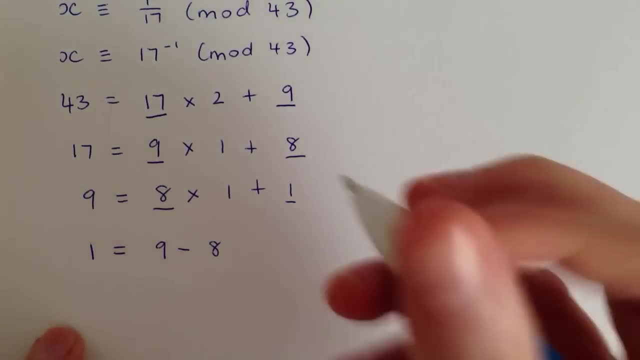 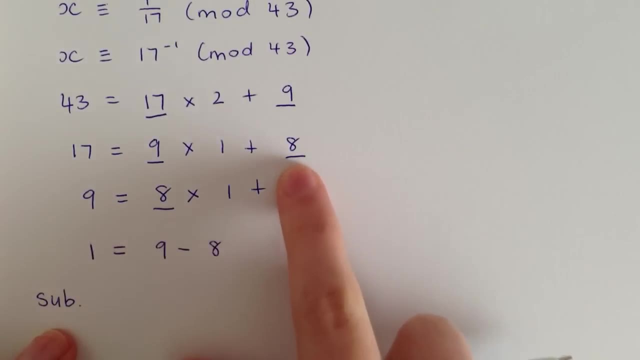 leave that off, because it's the same as saying 8.. Okay, so now we want to sub in. We've already worked with this equation, So we want to back up the Euclidean algorithm And we want to sub in this equation here. Now we want it. 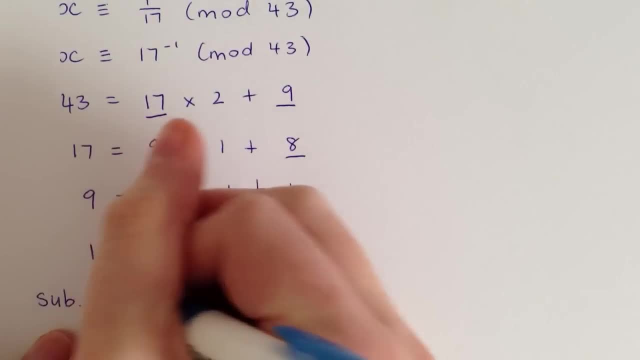 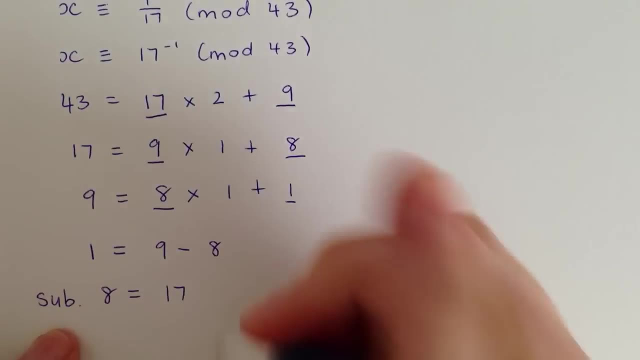 in terms of this number on the end, again So same as we did before. just take this 9 times 1 over the other side. So that gives us 17 minus 9 times 1 over the other side. So that gives us 17 minus 9, again times 1, but we can just leave it off because it's. 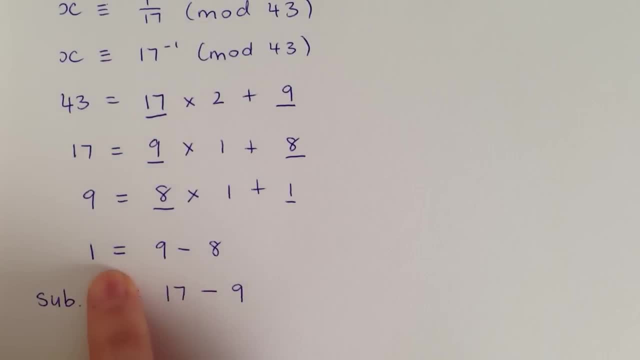 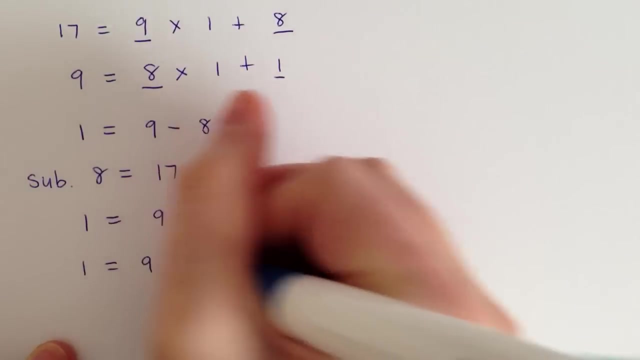 the same. So we want to sub this equation into this one just above it. So we'll get 1 equals 9 minus where there's an 8, you want to put this 17 minus 9.. And then we can just simplify that. A negative and a negative make a positive, And we can simplify that. 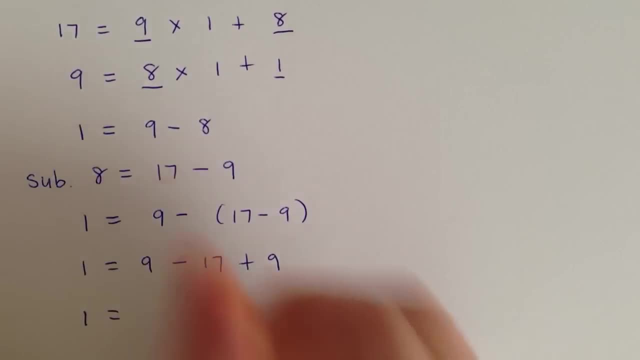 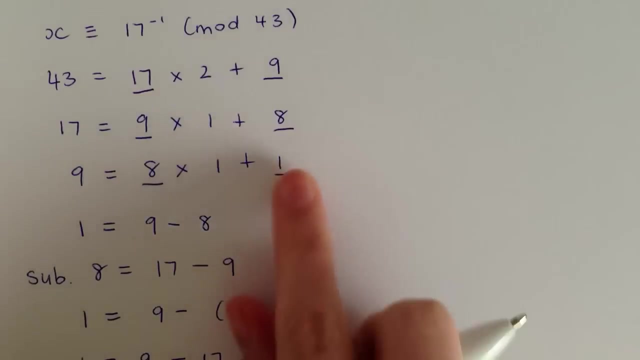 one again. We've got a 9 and a 9. So that makes 9.. And then we've got a 9 and a 9. And that makes 2 times 9.. And then minus 17.. Okay, so now we've already subbed in here this equation, So we want to go back up the 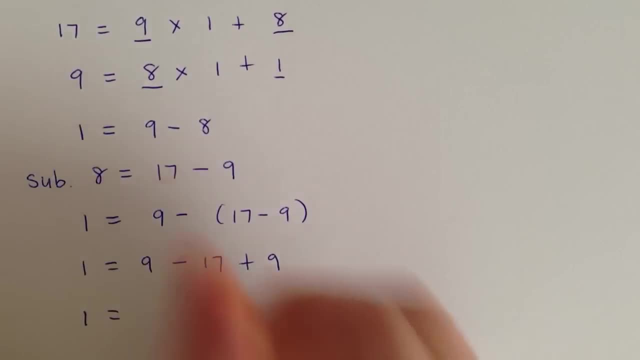 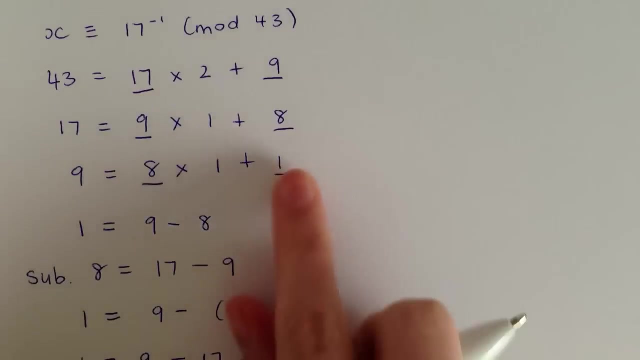 one again. We've got a 9 and a 9. So that makes 9 times 1 over the other side, And then that makes 2 times 9.. And then minus 17.. Okay, so now we've already subbed in here. 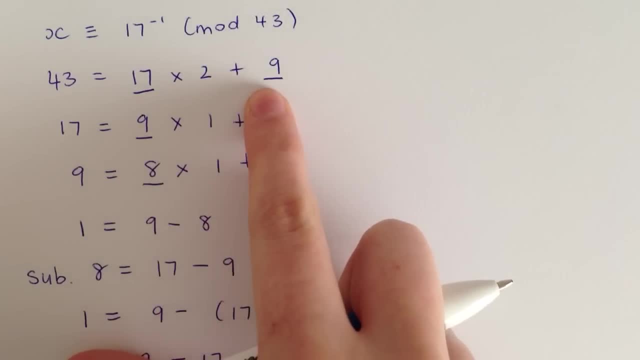 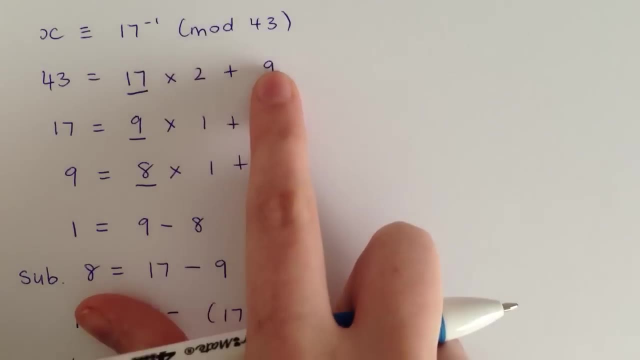 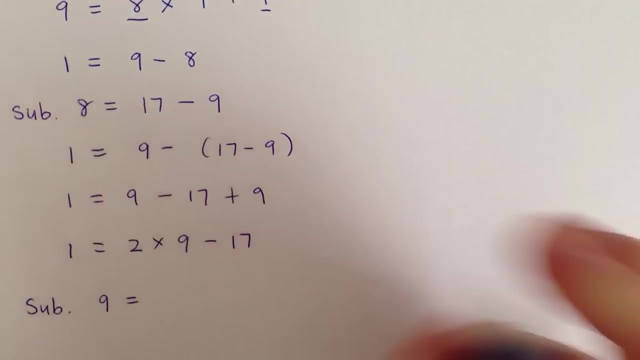 this equation. So we want to go back up the Euclidean algorithm And we want to use this one instead. So we want to sub that into what we've just done. So again, we want it in terms of this: 9 here, So that'll make it: sub 9 equals 9 times 1 over the other side, So that's. 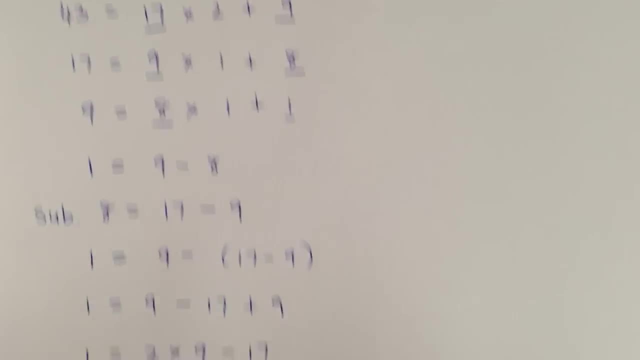 going to take this 17 times 2 over the other side, So we get 43 minus 17 times 2.. Now we want to sub this one into the one before it, So that makes 1 equals 2 times instead of. 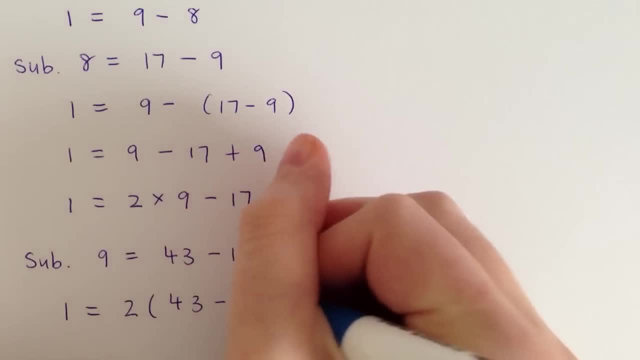 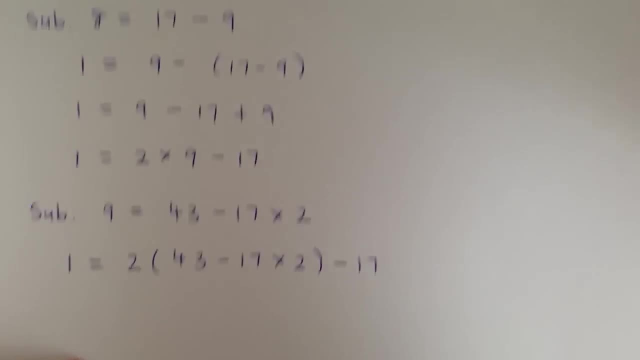 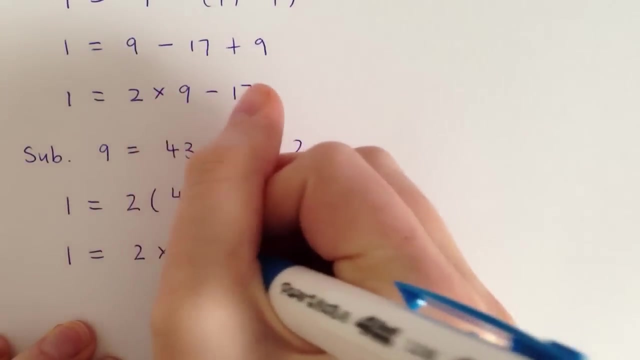 a 9,. we want to write this equation here, And then- don't forget this minus 17 as well. Okay, and then we can just expand that one Now. so we've got 2 times 43. And then, because this 17 is in the original equation, we want. 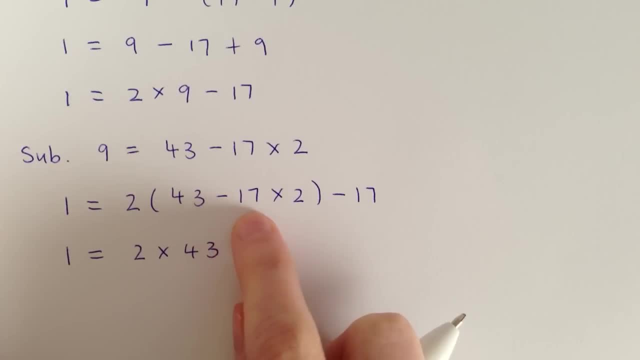 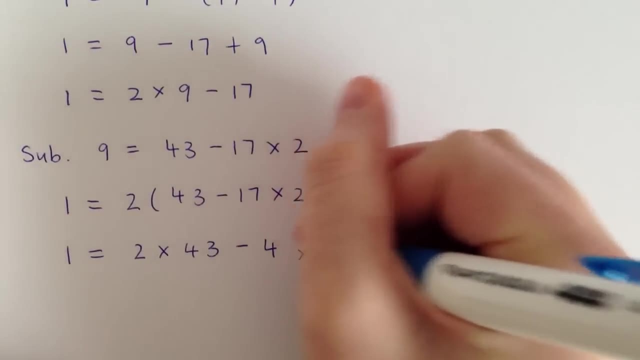 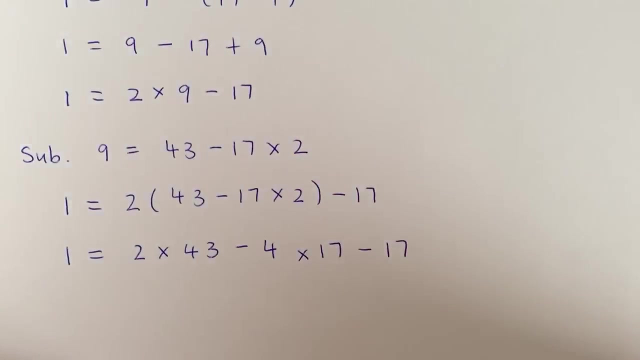 to keep it in terms of that 17.. So we've got negative 17 times 2, and then times 2 again. So that is the same as saying negative 4 times 17.. And then we also have this extra minus 17.. 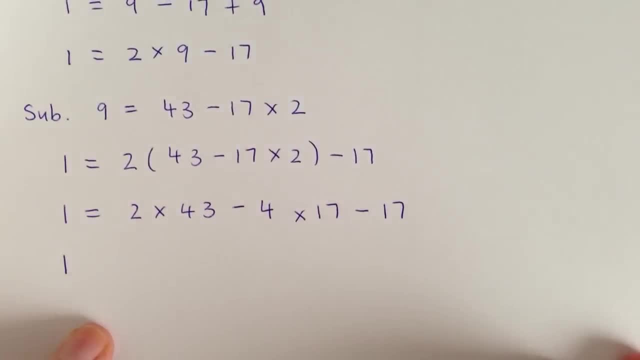 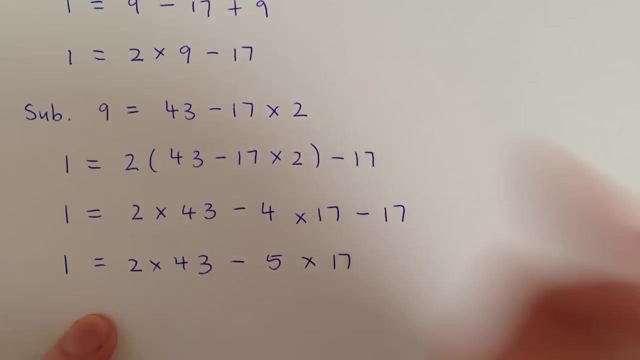 So we can simplify that again. So 2 times 43. We've got a negative 4 times 17, and a negative 1 times 17. So that's negative 5 times 17.. Okay, and so we've got our equation in terms of 43 and 17.. Now, because the original question 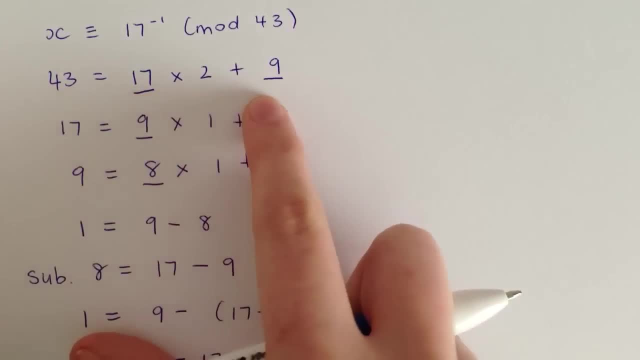 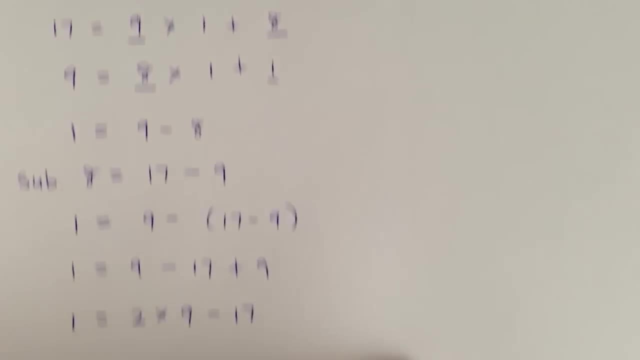 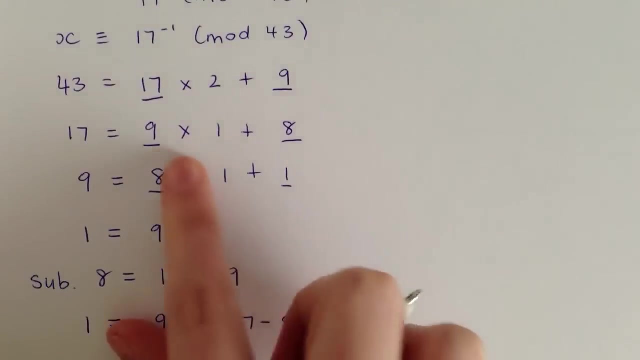 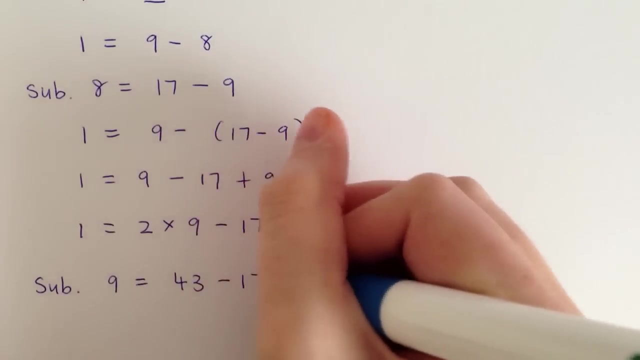 Euclidean algorithm And we want to use this one instead. So we want to sub that into what we've just done. So again, we want it in terms of this: 9 here- So that'll make it sub 9- equals 2 over the other side. So we get 43 minus 17 times 2.. Now we want to sub this one into 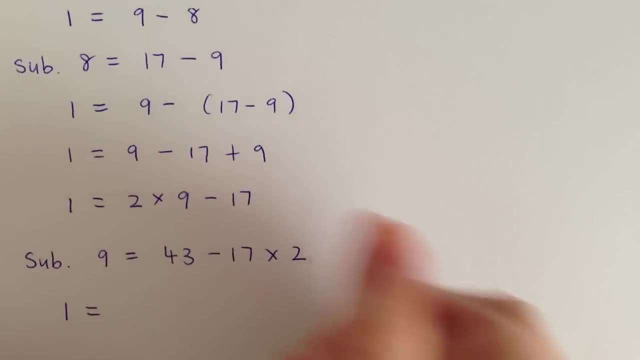 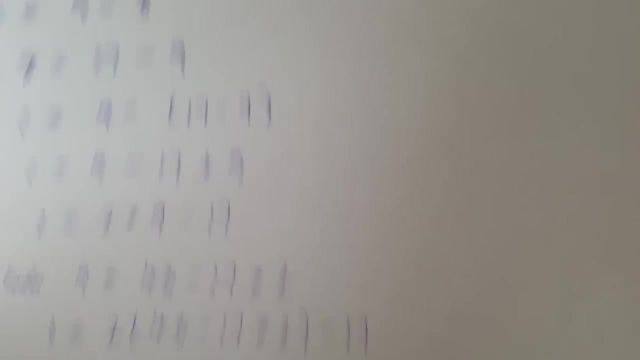 the one before it. So that makes 1 equals 2 times instead of a 9,. we want to write this equation here And then- don't forget this minus 17 as well. Okay, and then we can just expand that one in. So we've got a 9 minus 17 times 2 over the other side. So we 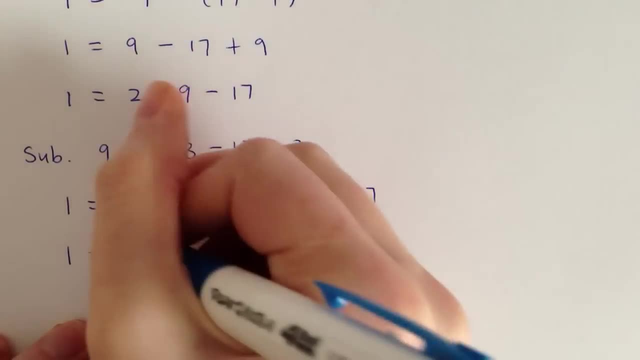 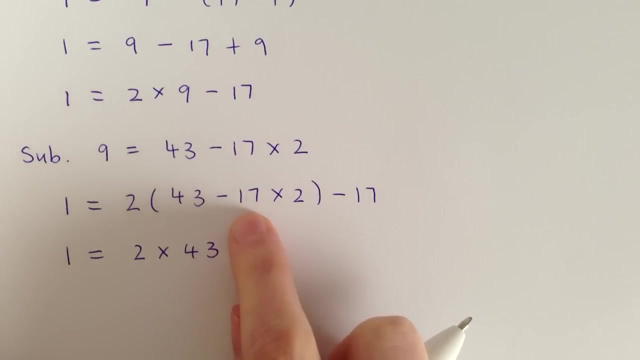 want to keep that one out. So we've got 2 times 43. And then, because this 17 is in the original equation, we want to keep it in terms of that 17.. So we've got negative 17 times 2, and then times 2 again. So that is the same as saying negative 4 times 17.. 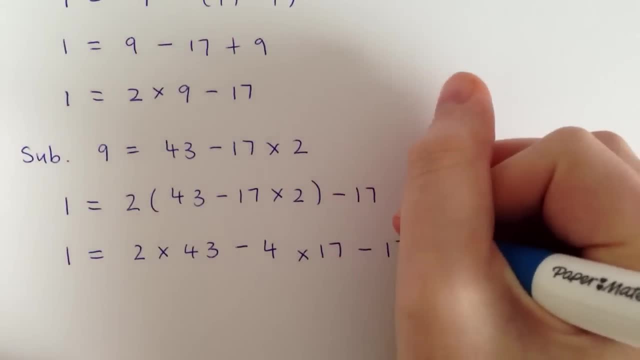 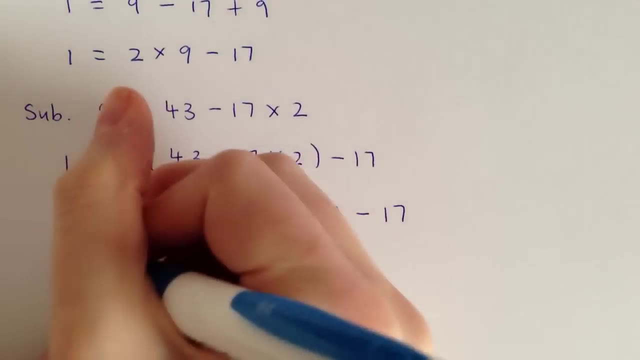 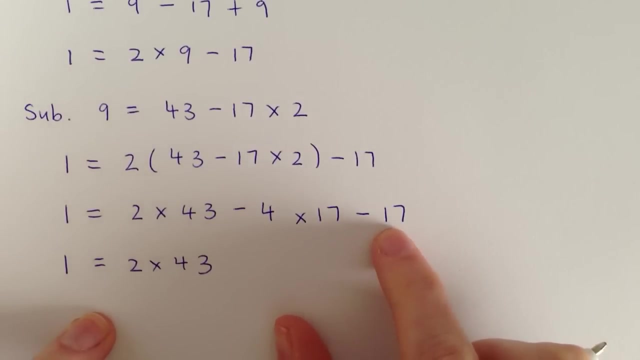 And then we also have this extra minus 17. So we can Simplify that again: So 2 times 43. We've got a negative 4 times 17 and a negative 1 times 17.. So that's negative 5 times 17.. Okay, and so we've got our equation in terms. 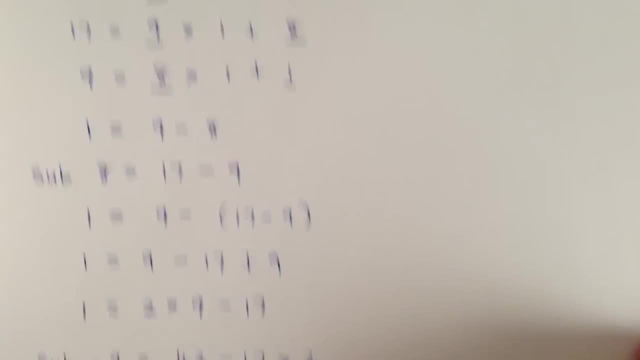 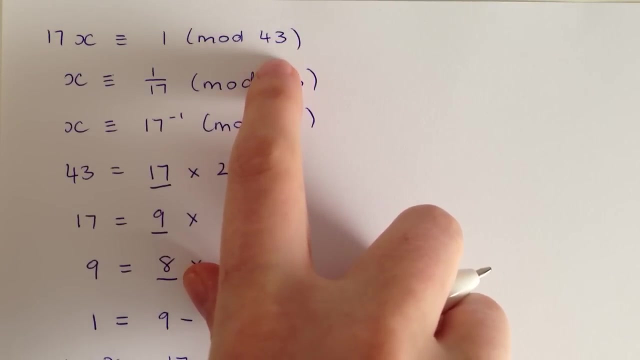 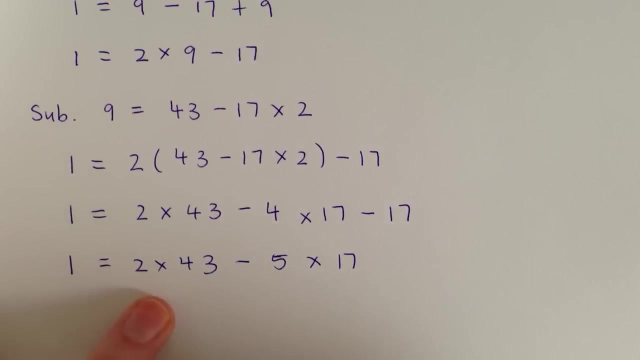 of 43 and 17.. Now, because the original question was mod 43, anything times 43, mod 43 is going to be 0. so in this bottom equation here, when we have 2 times 43 there it's only it's gonna equal 0 because it's mod 43. 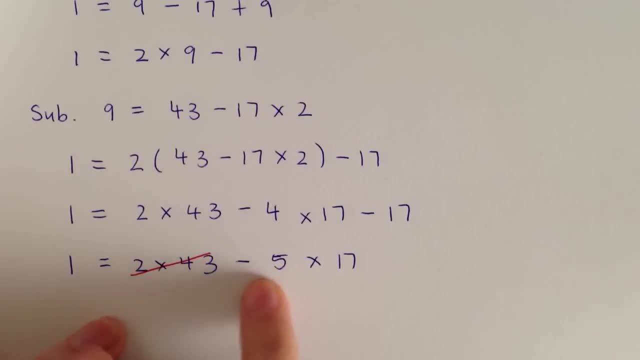 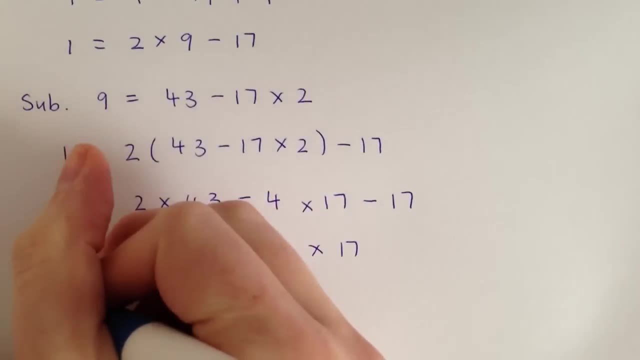 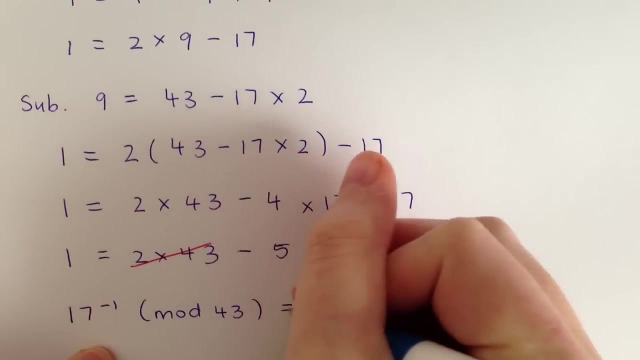 so we can just cross that out and then it's just whatever number is attached to this- 17 here, because that's what was in the original question. so we've got 17 to the power of minus 1 mod 43 is equivalent to negative 5. now we want that between: 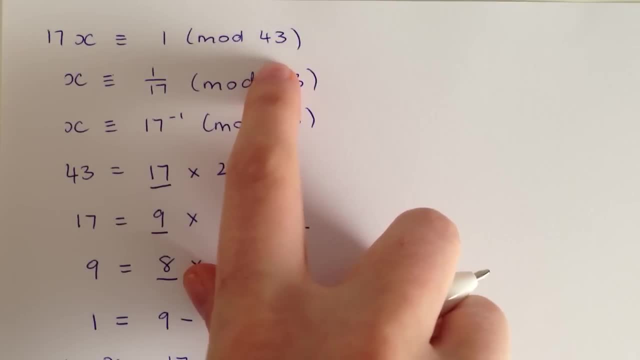 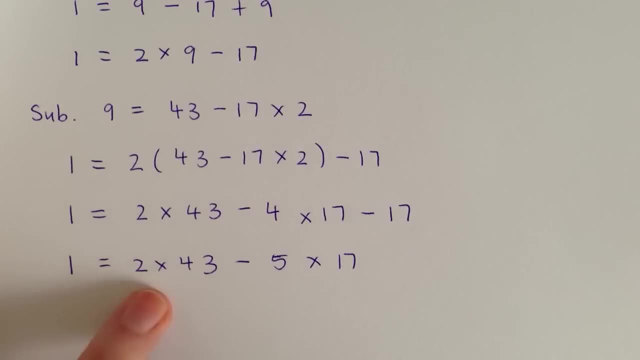 was mod 43, anything times 43,, mod 43, is going to be 0. So in this bottom equation here, when we have 2 times 43, there it's only it's going to equal 0 because it's mod 43. So we can.